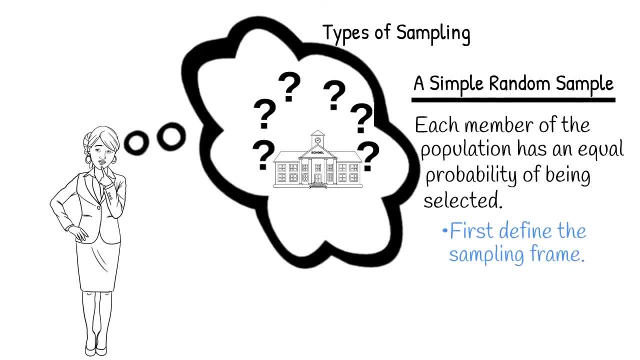 is drawn. So if the population she's interested in is a school, the sampling frame could be all the students registered in the school. Then she should design a method to select randomly from that frame. She could draw numbers from a bag. design a method using 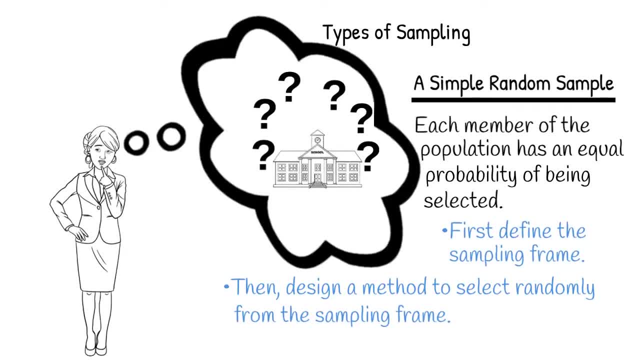 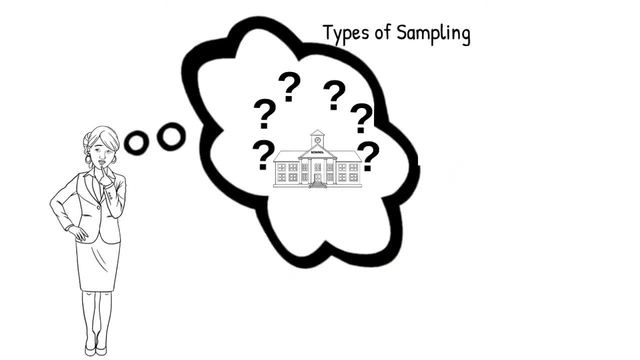 number generation or use another method of her choice, as long as her selections are truly random. While Kate likes the idea of using this method to collect data, what if it's important that she surveys the same number of men and as women, or if she wants race in her sample to be represented in? 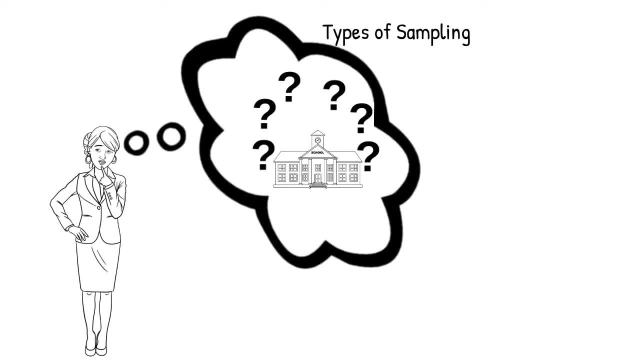 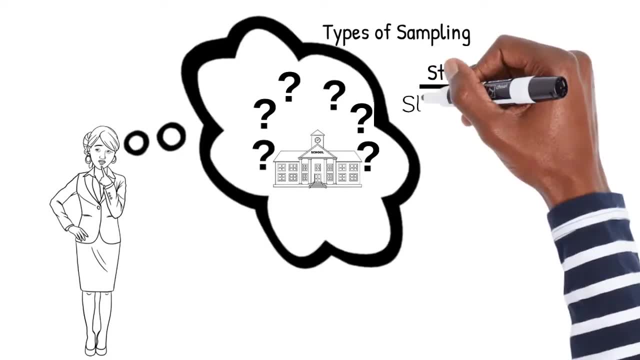 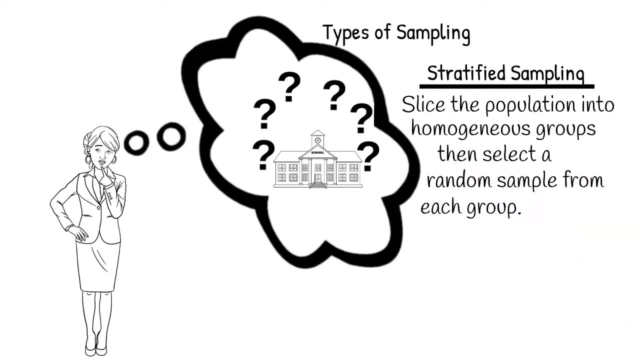 the same proportions as the population. In those and similar cases, a stratified sample might be a better idea. In stratified sampling we slice the population into homogeneous groups, then select a random sample from each group. Each homogeneous group is called a stratum. put together the 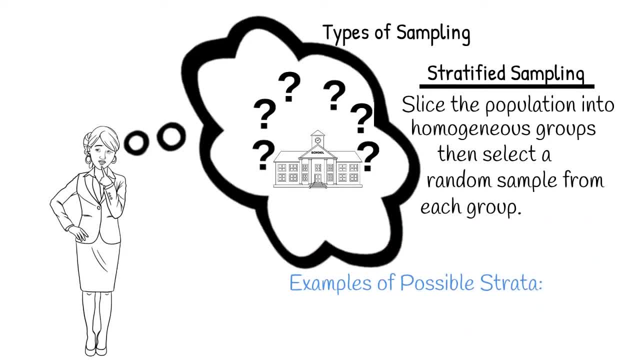 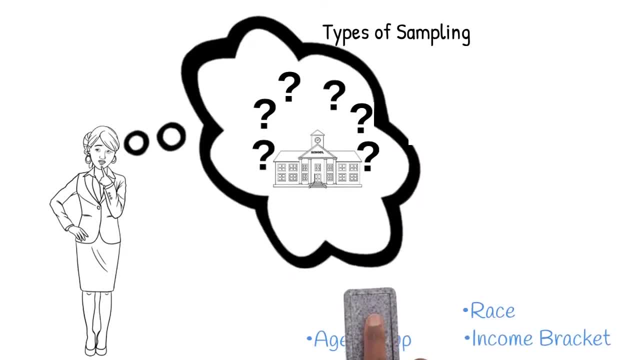 groups are called strata. Examples of common strata are gender, race, age group and income bracket, and then your amount of files. The loincloths, fingerprints and information w cat are operated in a model. Another option for collecting data is cluster sampling. 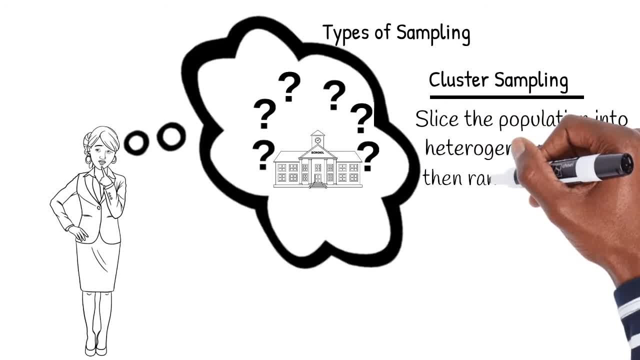 Kate can slice the population into heterogeneous groups, then randomly select a group or groups to perform a census on. The big difference between stratified sampling and cluster sampling is that in stratified sampling our groups are homogeneous- They share a characteristic, But in cluster sampling our groupings must be heterogeneous. 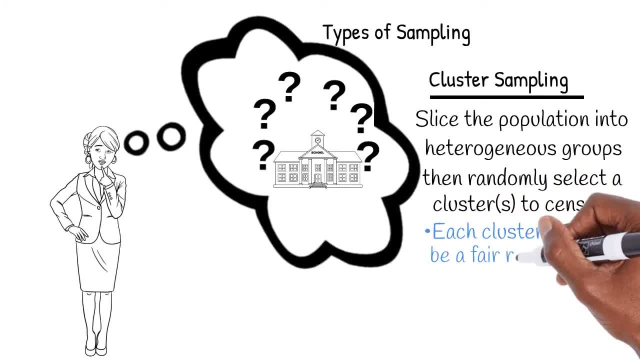 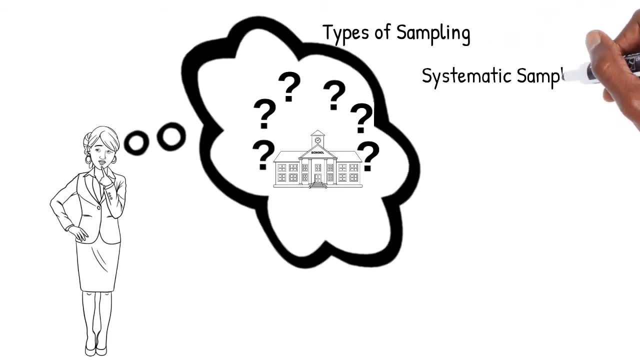 This mix of characteristics in each cluster should be a fair representation of the population. This is a good option for sampling because it is more practical than doing a census of the entire population. Another option for collecting data is systematic sampling. This gives Kate the opportunity to design her own approach for randomly selecting a. 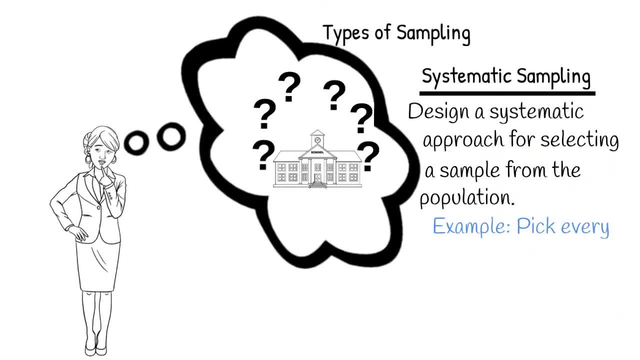 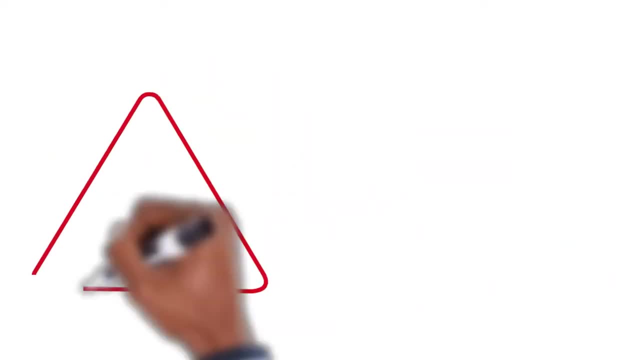 sample from the population. For example, she could list names alphabetically, then pick every ten things that are related to the population. To make this truly random, the first number selected should be randomly selected. The sampling methods discussed so far all use the element of randomness to avoid bias.